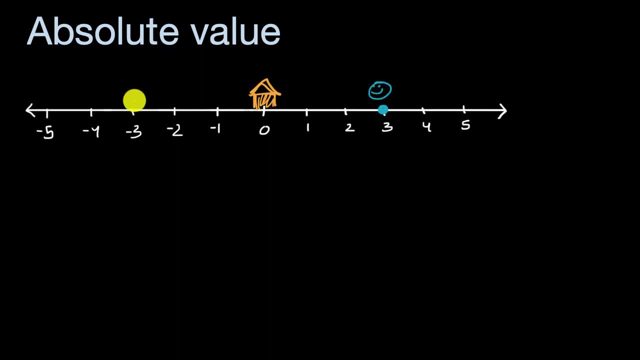 And that you live three miles to the left of the school. So this is where you would be three miles to the left, or maybe we could say that's to the west of the school. Now you could say that your position is at negative three miles relative to the school. 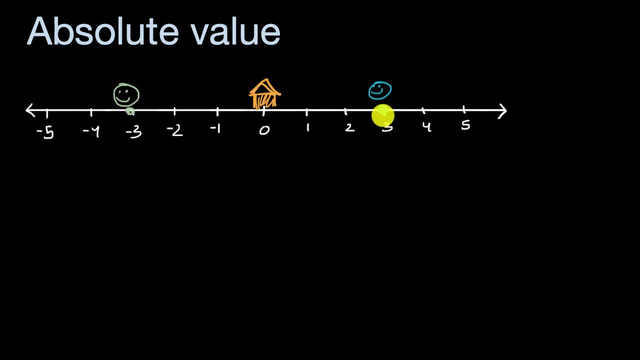 and my position is at positive three miles relative to the school. But what we might care about is just how far are we from the school, And so there you could say: well, we're each exactly three miles from the school. You're three miles from the school. 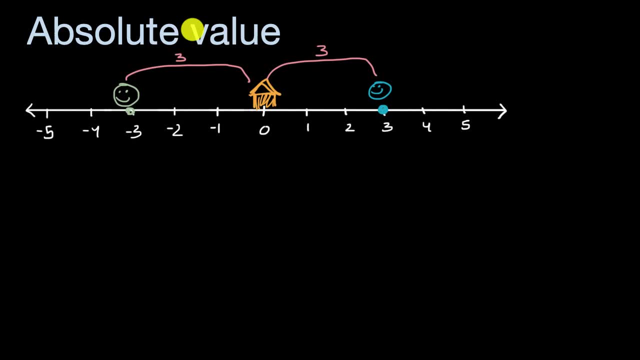 and I am three miles from the school, And that's what absolute value is actually trying to get at. So, for example, your position is negative three, But if we were to take the absolute value which you denote by these two straight up down bars, 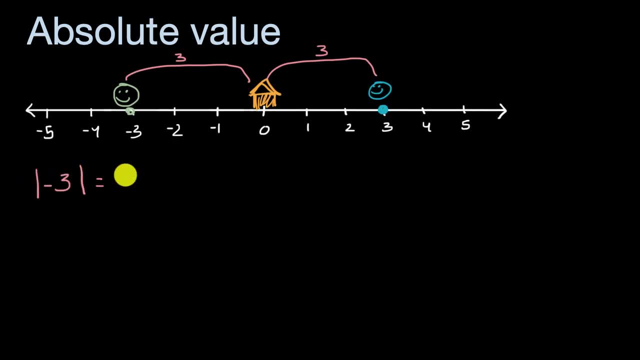 around the number. then we say: that's just going to be your distance from zero, which is just going to be three miles. Similarly, my position is at three miles positive three miles. The absolute value of that is going to be. 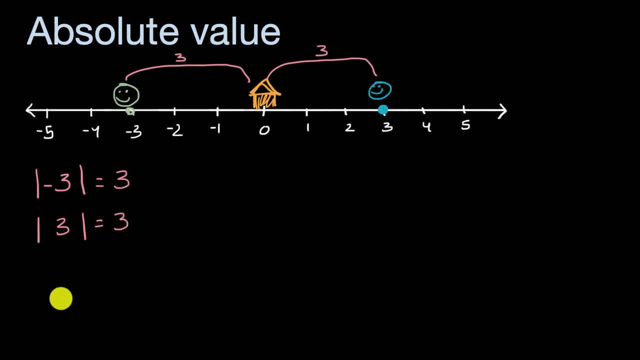 drum roll, please. it is going to be three as well. You might already see a pattern: If you're taking an absolute value of a negative number, you get the number without the negative, And if you take the absolute value of a positive number, 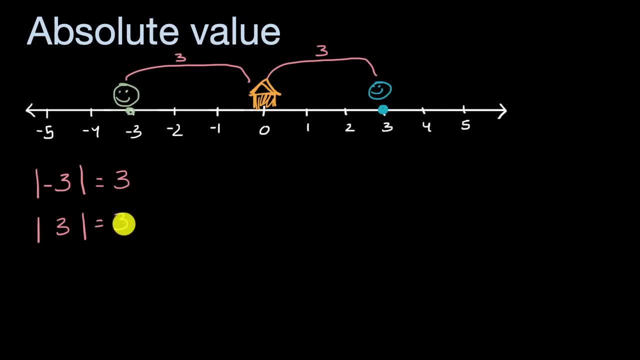 it just equals itself again. But the reason why that is the case is because we're just, we're just taking the absolute value of a positive number, it just equals itself again. We're just saying: how far is that thing from zero? 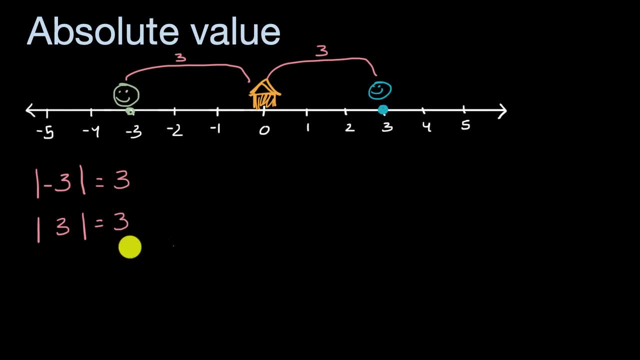 Let me give another example. Let's say that we have some type of a cruise ship and that's the water right over there. This is the cruise ship. Let me draw it. This is big cruise ship, nice and big one, has water slides on it and whatever else. 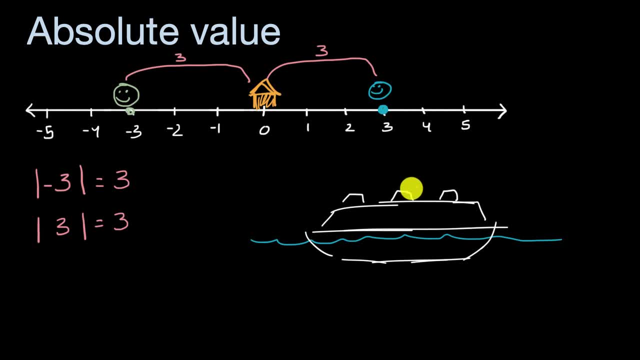 whatever you would expect from a huge cruise ship. And let's say we think about the height of where the different floors are in the ship and a natural place to think about is based on where the sea level is, So we call that height zero. 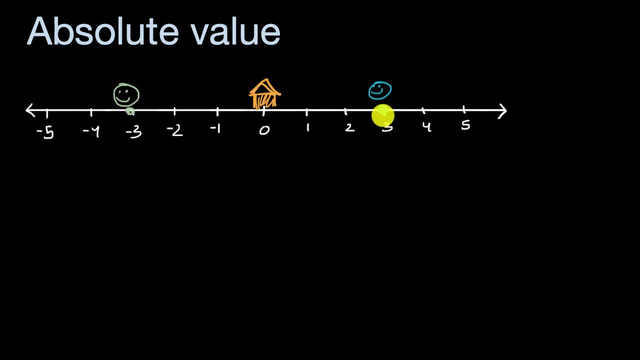 and my position is at positive three miles relative to the school. But what we might care about is just how far are we from the school, And so there you could say: well, we're each exactly three miles from the school. You're three miles from the school. 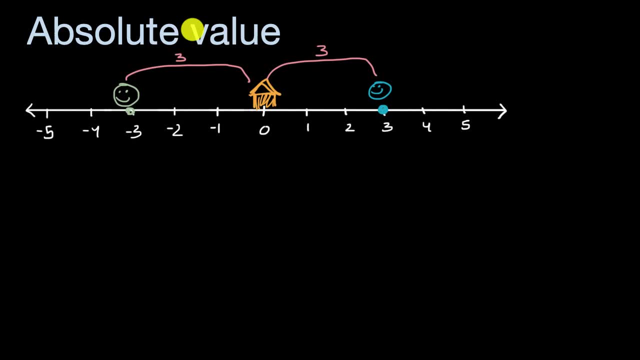 and I am three miles from the school, And that's what absolute value is actually trying to get at. So, for example, your position is negative three, But if we were to take the absolute value which you denote by these two straight up down bars, 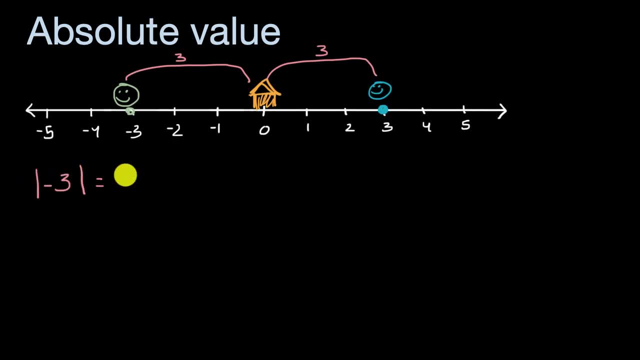 around the number. then we say: that's just going to be your distance from zero, which is just going to be three miles. Similarly, my position is at three miles positive three miles. The absolute value of that is going to be. 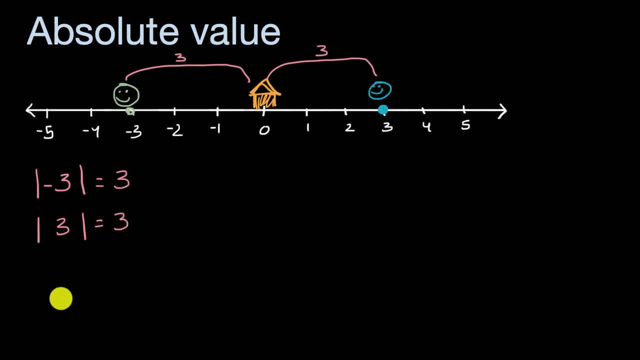 drum roll, please. it is going to be three as well. You might already see a pattern: If you're taking an absolute value of a negative number, you get the number without the negative, And if you take the absolute value of a positive number, 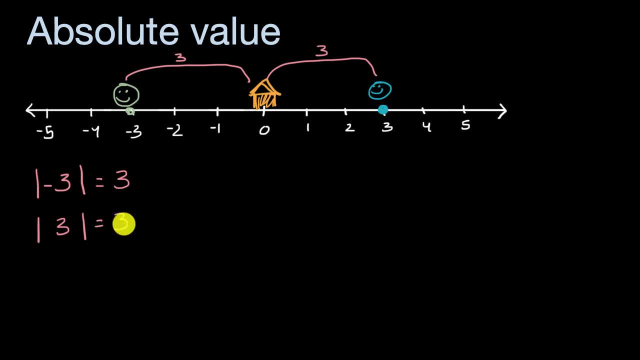 it just equals itself again. But the reason why that is the case is because we're just saying how far is that thing from zero? Let me give another example. Let's say that we have some type of a cruise ship and that's the water right over there. 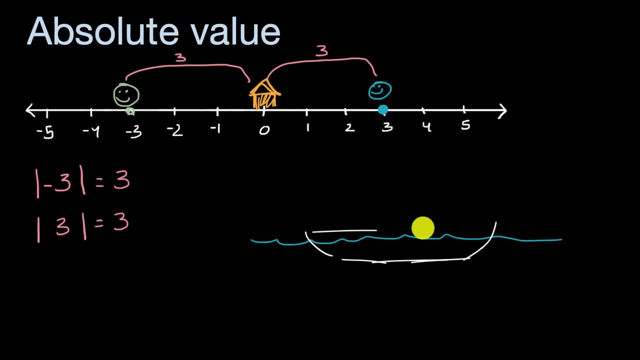 This is the cruise ship. Let me draw it. This is a big cruise ship, nice and big one, has water slides on it and whatever else. whatever you would expect from a huge cruise ship. And let's say we think about the height. 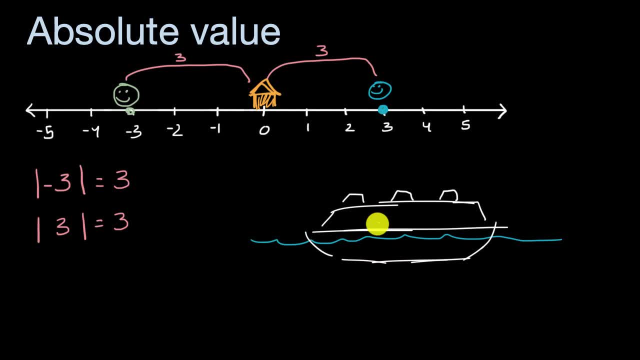 of where the different floors are in the ship, And a natural place to think about is based on where the sea level is, So we call that height zero. Now there's this big waterfall pool type thing up here. Let's just say it's a pool, for simplicity- on the roof. 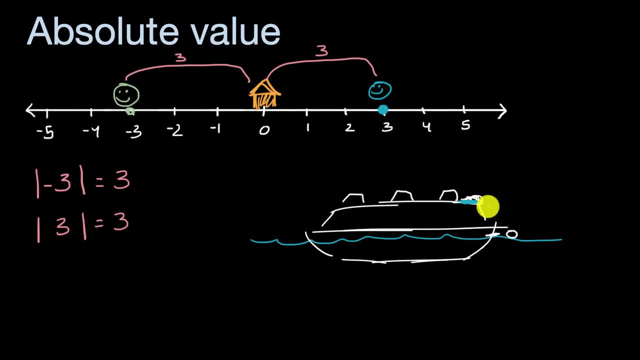 And let's say that that is at an altitude of 80 feet, So we would call that at positive 80 feet. And let's say the engine room is right over here And if you wanted to know its position, its height, well, it is going to be below zero.